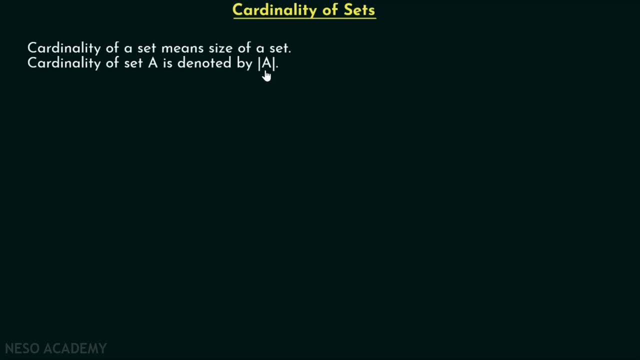 As simple as that. If there are n distinct elements, then the cardinality of the set will be n. Okay, Also, I am talking about finite sets. I am not talking about infinite sets. Okay, We will discuss the cardinality of infinite sets later. 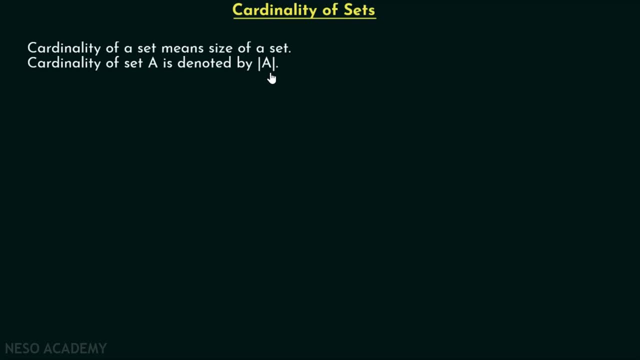 It is quite an interesting topic. We will discuss it later. Okay, Now here is one example: A set of all odd positive integers less than 10.. Obviously, this is a finite set, right? We are talking about all odd. 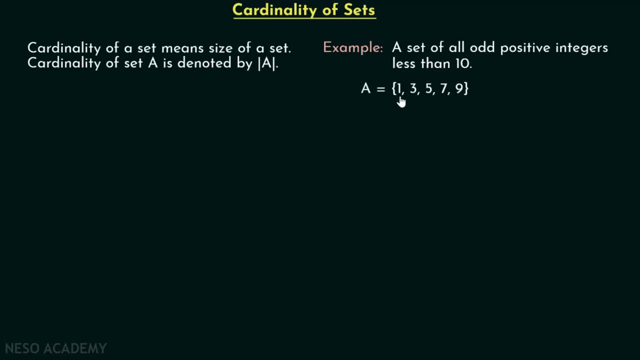 Odd positive integers less than 10.. Here is how it looks like. We have 1,, 3,, 5,, 7,, 9.. I am representing this set by A capital A, So it is clear that cardinality of this set is 5.. 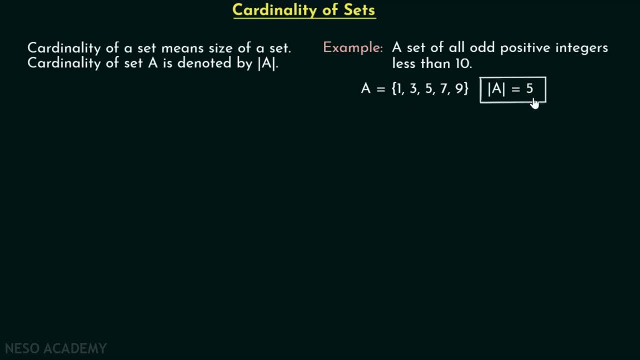 There are total 5 elements in this set. right, Let's discuss one more example. Cardinality of a null set is 0.. Very simple, Because there is no element in null set. That is why cardinality of null set is 0.. 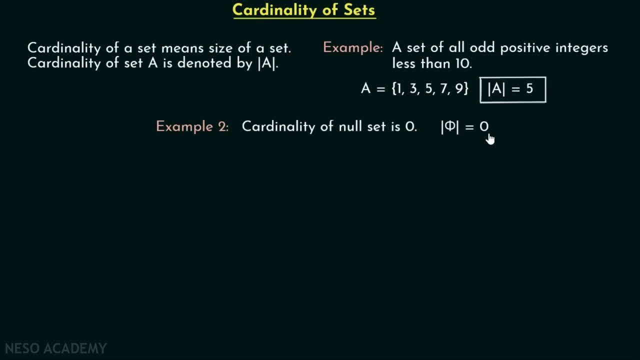 Or, in other words, we can say that cardinality of 5 is 0.. Now in this presentation, we will also discuss one more example. We will discuss one gate problem, which is very important, Although it is very simple. 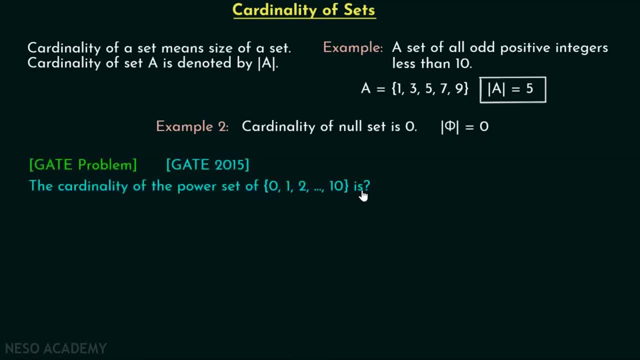 but it is important- The cardinality of the power set of this set is- This question has been asked in GATE 2015.. We have to find out the cardinality of the power set of this set. Let's say this set is represented by capital A. 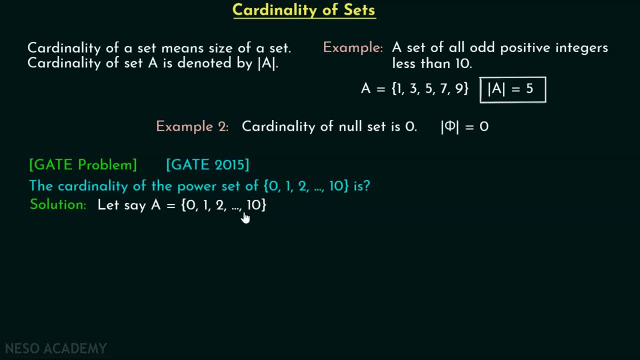 Okay, Now I would like to ask this question: How many elements are there in this set? You might answer this: there are total 10 elements, But please note that this series is starting from 0 and not from 1.. 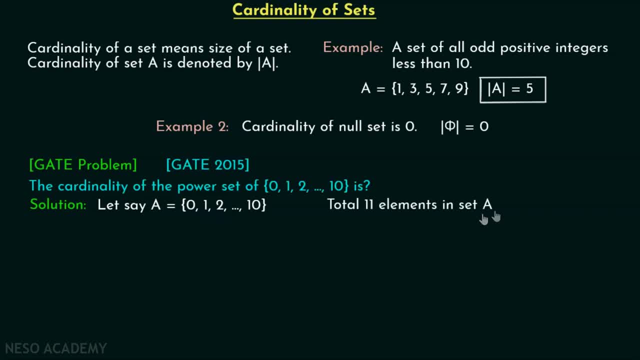 That is why there are total 11 elements. There are total 11 elements in set A. It might be possible that you make this mistake, that there are total 10 elements in this set, But please note that there are 11 elements in this set. 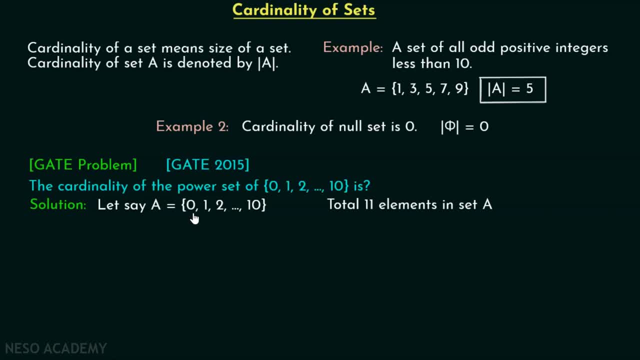 because the series is starting from 0 and not from 1.. That is why total 11 elements are there in set A. Therefore, it is clear that power set of A must have 2 to the power 11 elements. Thus cardinality of power set of A must be: 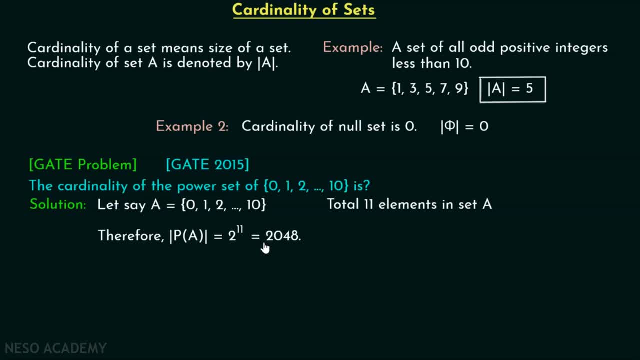 2 to the power 11,, which is 2048.. Isn't that so? Because there are 11 elements in set A, so cardinality of power set of A must be 2 to the power 11, which is 2048..